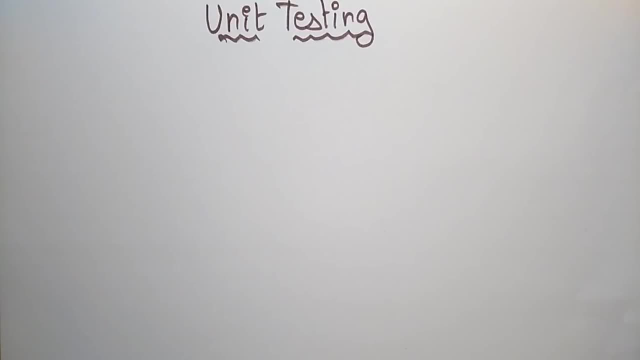 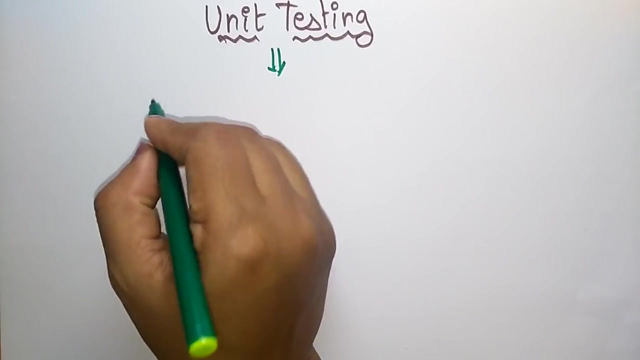 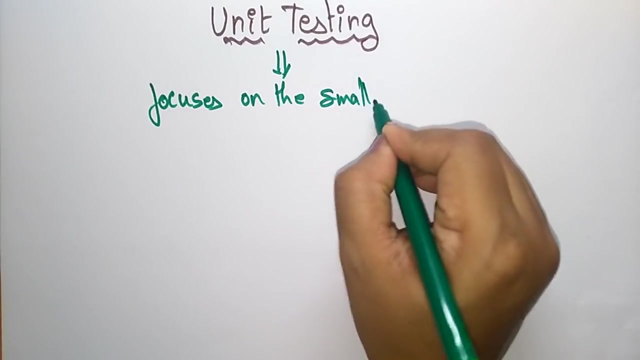 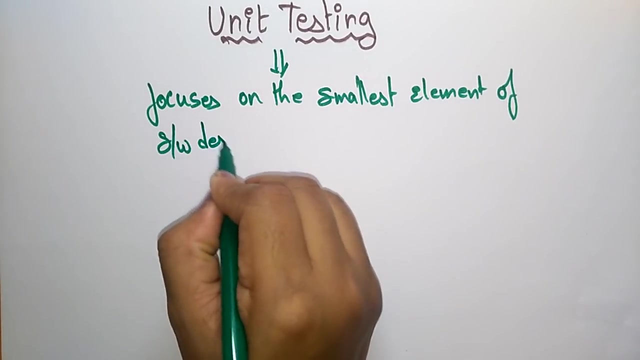 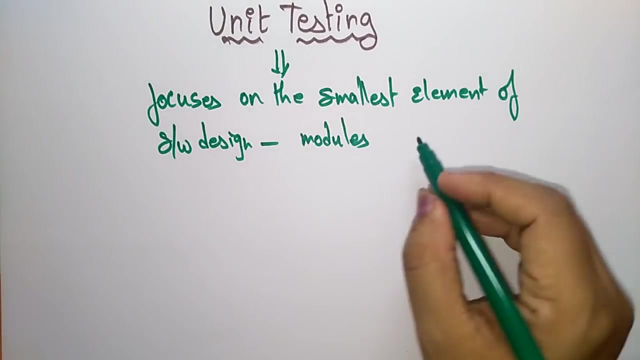 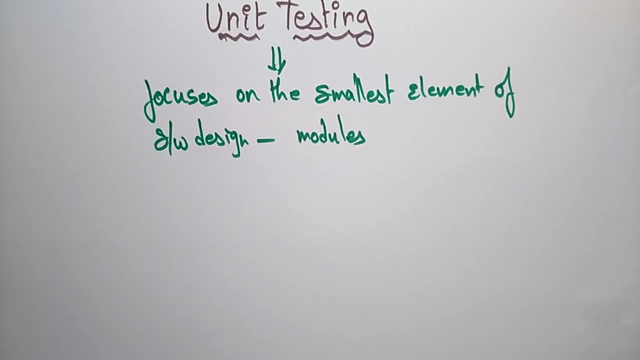 Hi students, coming to the next topic, that is, the unit testing. So the unit testing is mainly focused on the smallest element of software design. It focuses on the smallest element of software design, So that is like modules. It is focused on the modules or software components like that, So means it's just focusing on the small units. The complete structure is divided into different, different levels, So it is taking on the smallest element in the software design and try to test on that smallest unit Again. after that it integrated to the main next level module and again they tested. like that. 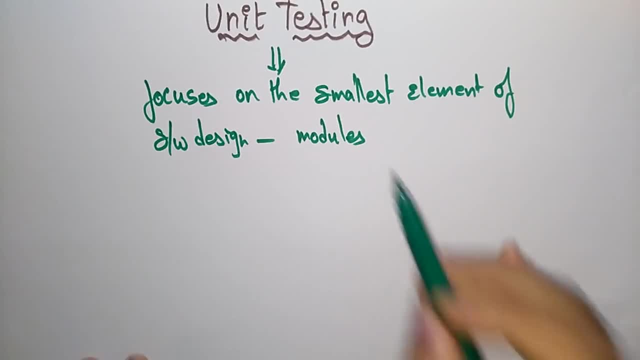 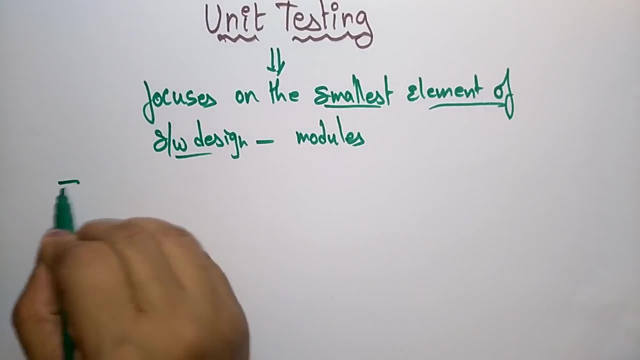 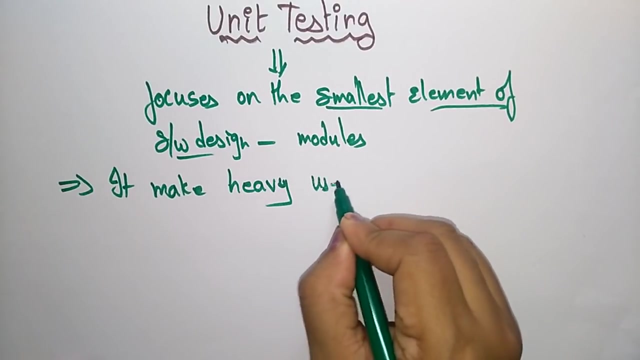 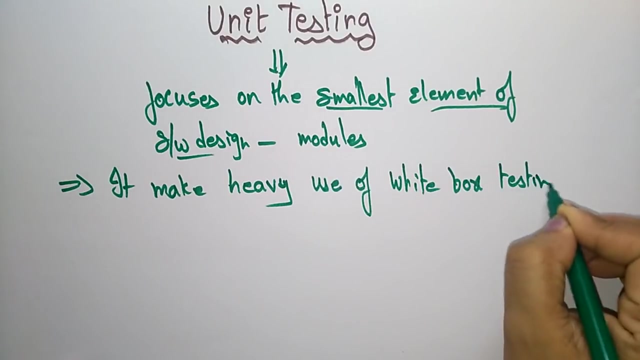 So the here, the unit testing, is only focused on the smallest element of the software design, So it make heavy use of the main thing is it make it make heavy use of white box testing. So actually the white box testing I will explain in the coming videos. But white box testing is mainly focused on the internal structure of the structure of the software. 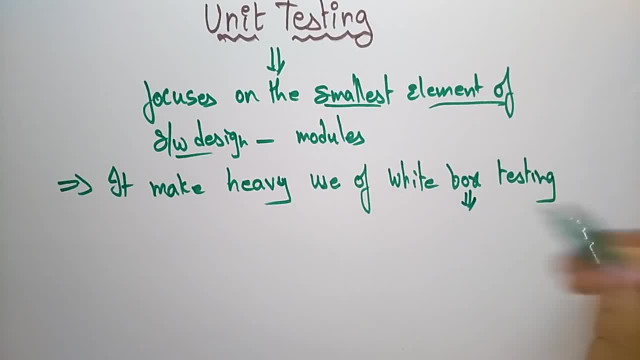 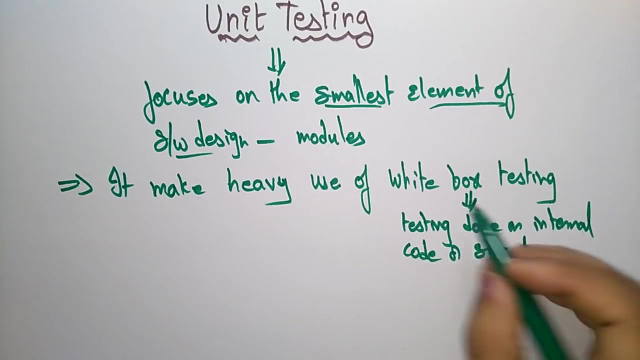 Module means completely. it is a testing on testing done on internal structure, internal code, internal code or structure. So unit testing means it is the smallest element. So if you want to test that smallest element you need the white box testing methodology. If you follow the white box testing methodology, 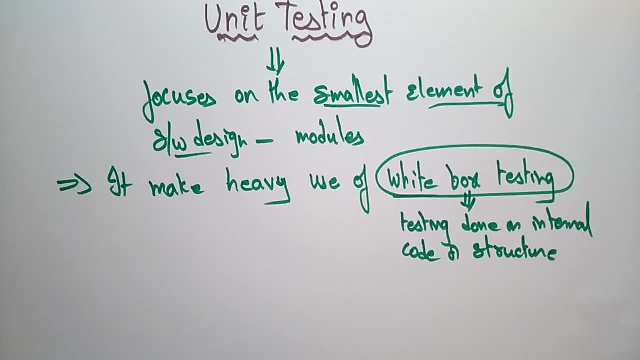 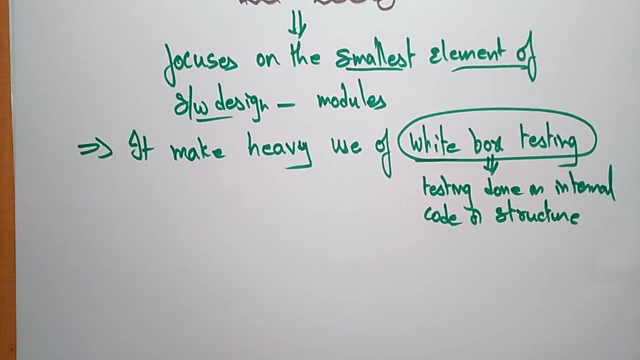 Then you can find out if any error is occurred or not. you can easily find out. the white box testing is nothing but is a testing done on internal code or a structure. Okay, So mainly the unit testing will use the white box testing methodology. So unit testing is a smallest testable parts of an application, called as units and are tested independently. So you have to be remember that here the testing will be done on the individual parts of the application. 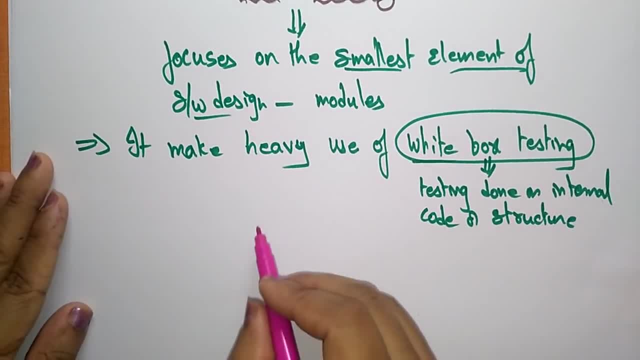 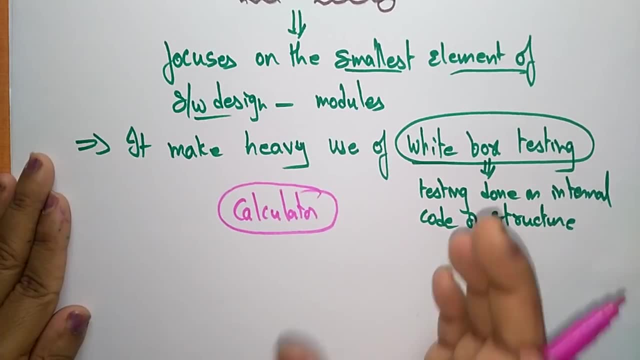 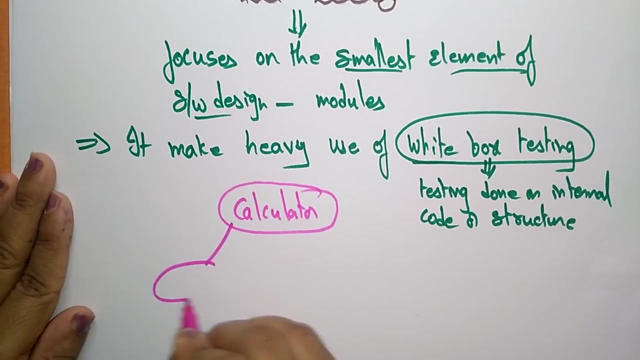 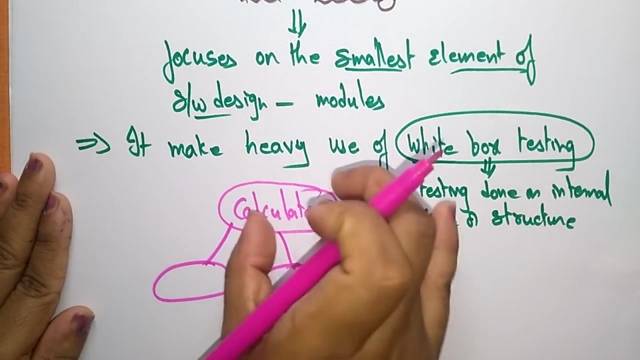 So you have to be remember that here the testing will be done on the individual units independently. Let me take an example. that is a calculator, So the calculator is one of the product. let us take: it is one of the product, So this complete system, the calculator, is a system. this system, I divided into subsystems, means the sub modules. So rather than working on a complete module, I divided the module into units, a small units. So that is, I am doing the operation. 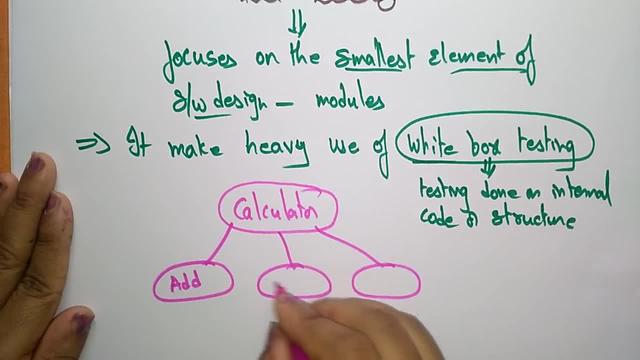 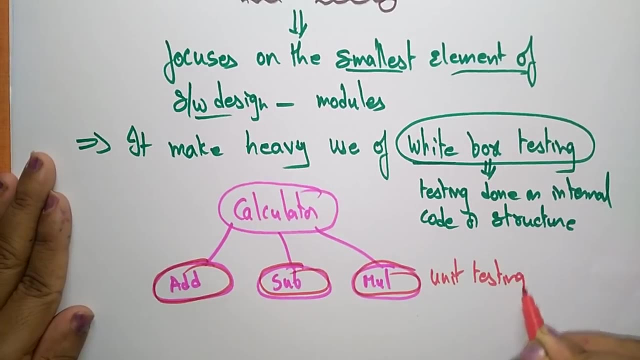 So I am checking the operations: is the addition is working properly or not, Subtraction, multiplication is working or not. So the testing that is done on this individual modules- you call it as unit testing. So how I am going to test this individual modules. So this test has to be done independently. 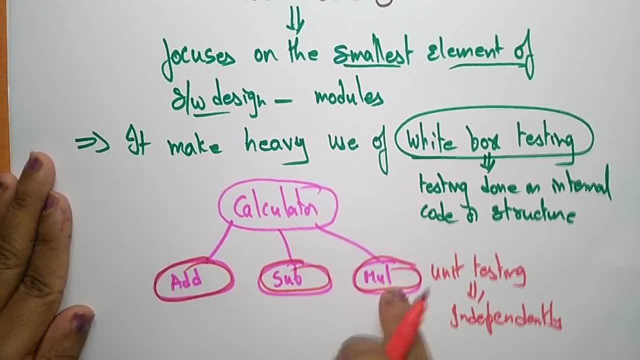 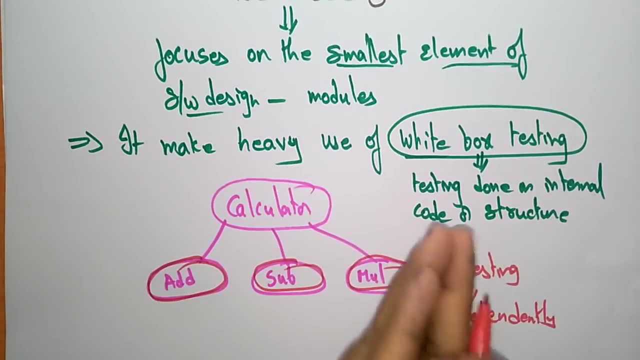 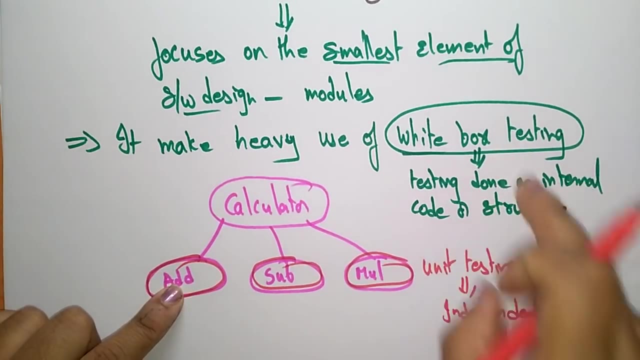 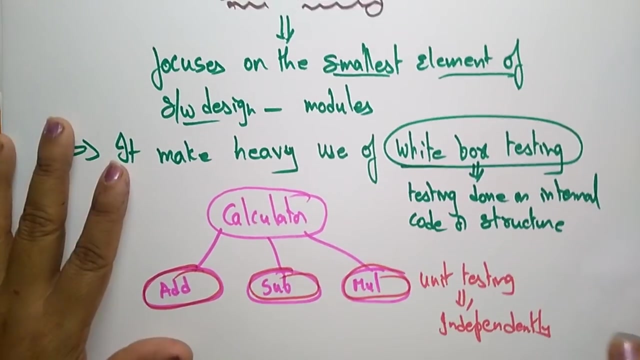 Okay Means there is no difference, dependency relation between these units. So addition is not dependent on subtraction and subtraction is not dependent on multiplication. So every module, every unit is tested independently. So this unit testing can be taken the help of methodology of white boxing testing, The testing that can be done in an internal code. So this is about unit testing. Let me explain some more example with. let us take any software engineering. 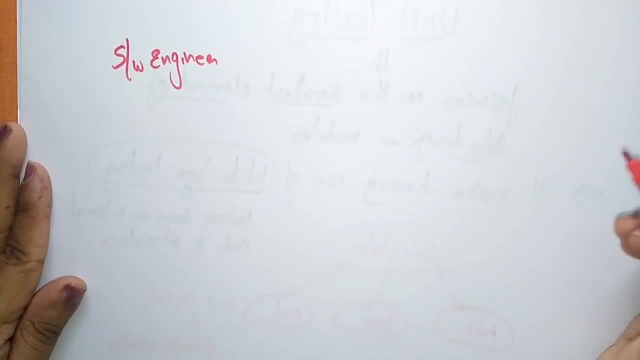 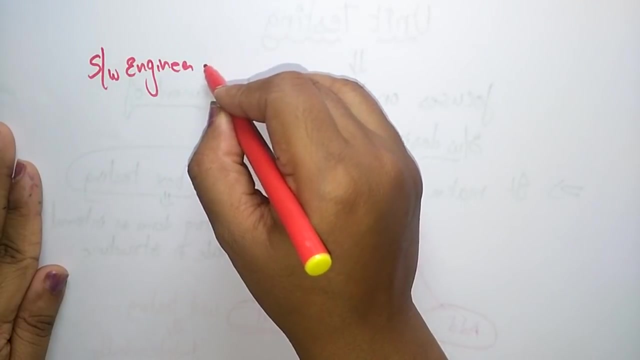 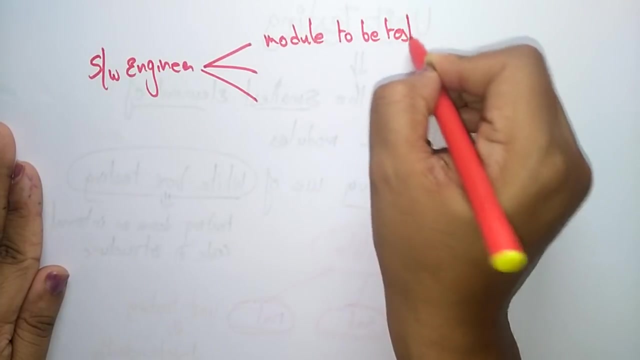 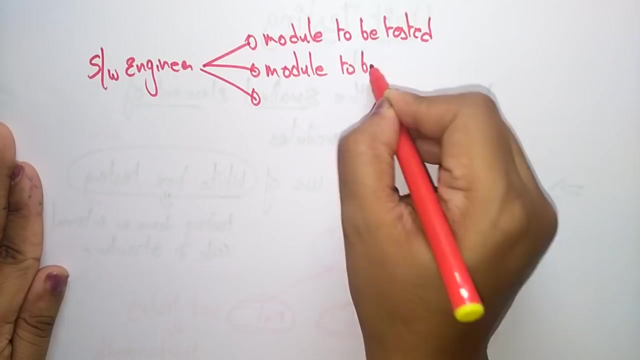 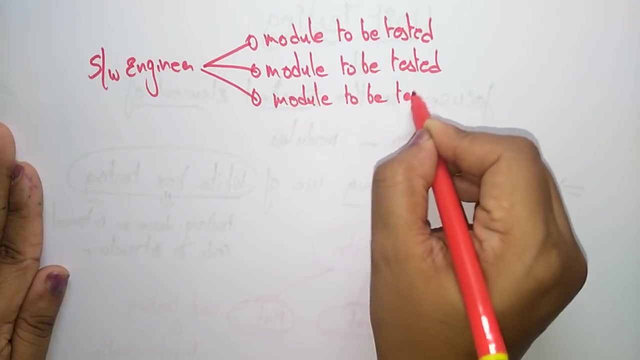 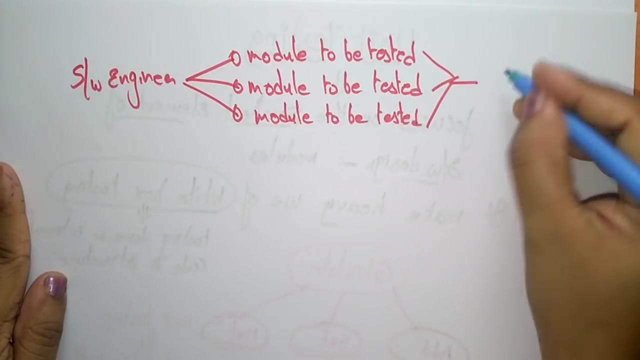 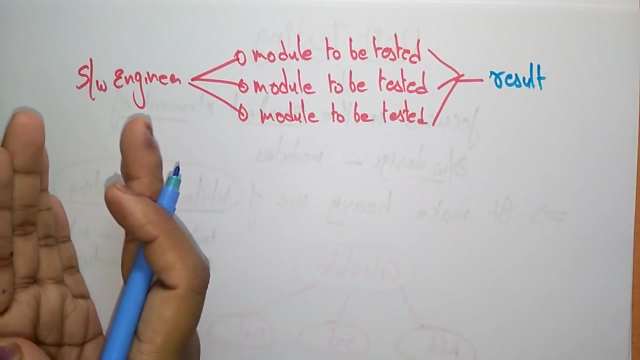 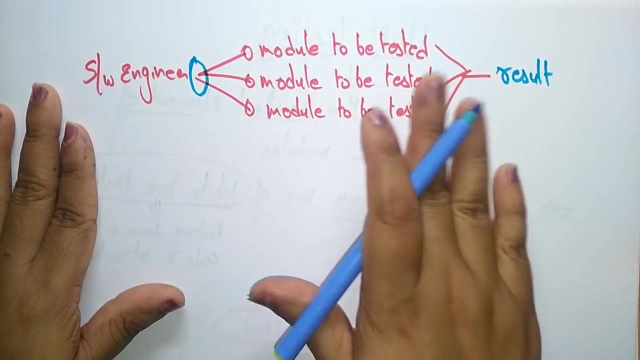 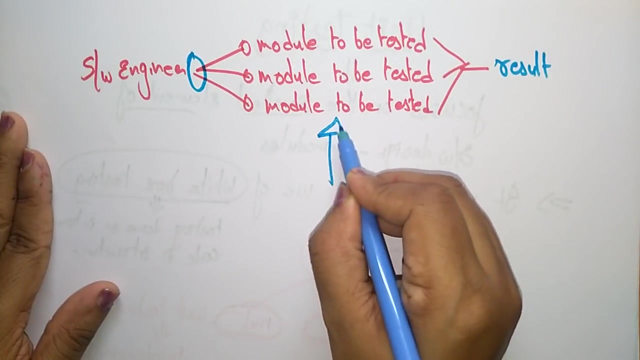 Okay. so the software engineering divide the product or modules into different modules. means sub modules, module to be tested. Each module he divided into modules and here the each module to be tested. So after testing the each module all has to be integrated and then final result will be appeared. Result will be sent to the means. the output will be given to the customers, whatever it may be. So the software engineer has going to divide the complete system into modules and that modules has to be tested and then the result will be appeared. So this modules will be tested based on some testing. So after testing, the each module all has to be integrated and then final result will be appeared. Result will be sent to the means. the output will be given to the customers, whatever it may be. So the software engineer has going to divide the complete system into modules and that modules has to be tested and then the result will be appeared. So this modules will be tested based on some testing. So after testing, the each module all has to be integrated and then final result will be appeared. Result will be sent to the means. the output will be given to the customers, whatever it may be. So the software engineer has going to divide the complete system into modules, and that modules has to be tested, and then the 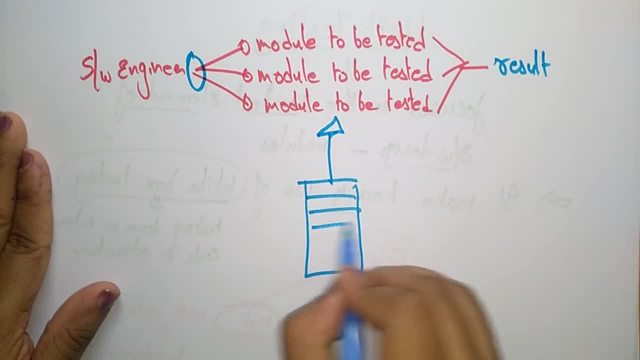 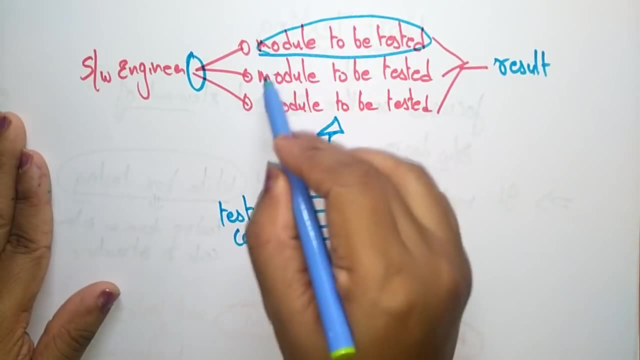 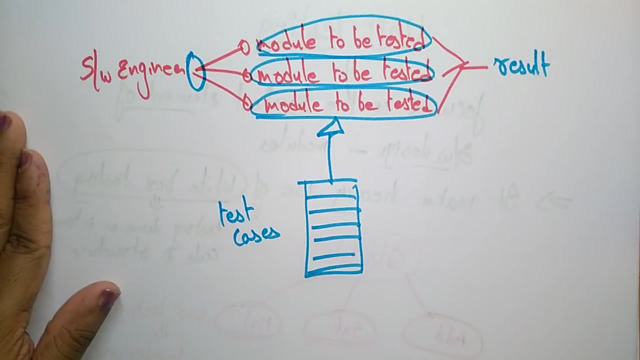 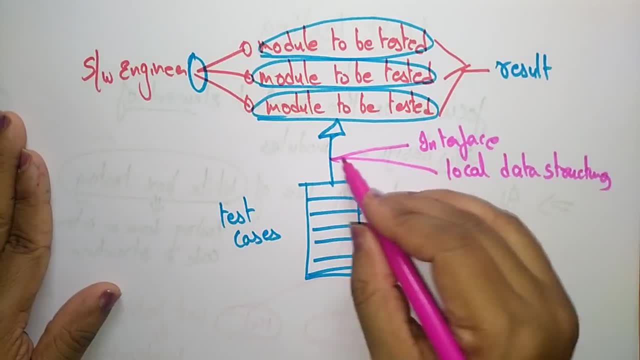 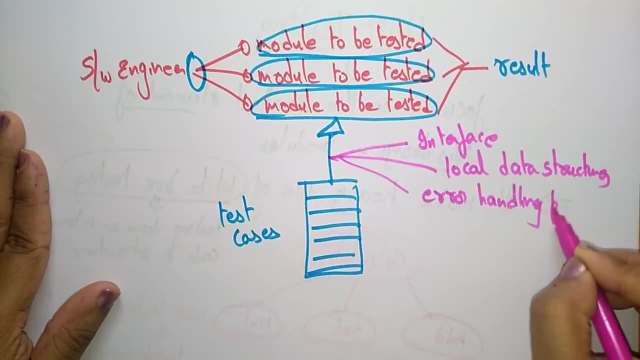 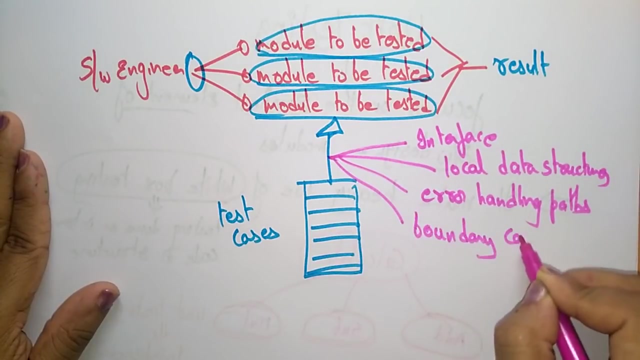 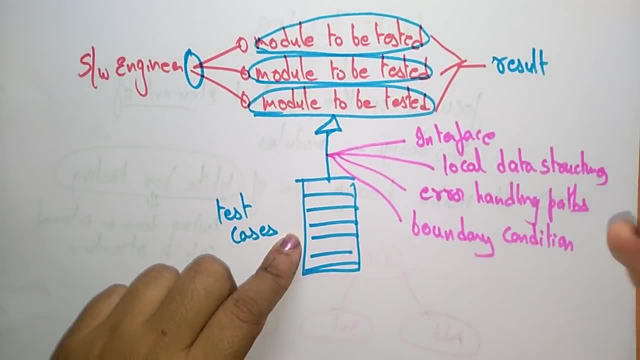 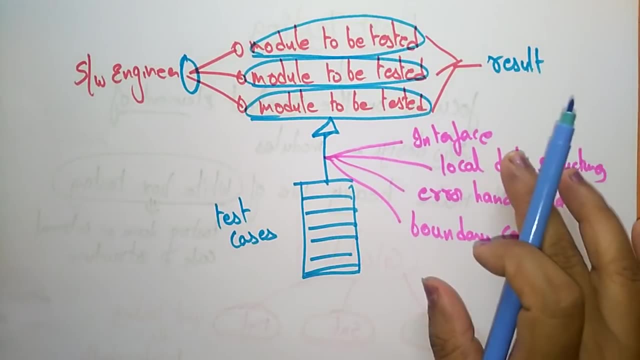 the interface consider. if you take the interface consideration, uh, here you have. you're going to check about number of input parameters, or equal to the number of arguments or not, and here the global variables definition is consistency or not. that's all comes under the interfaces. so on that. 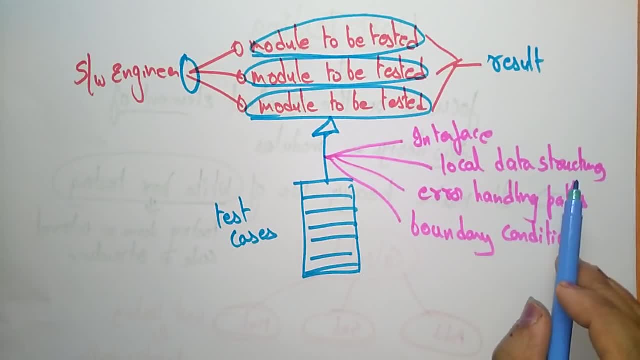 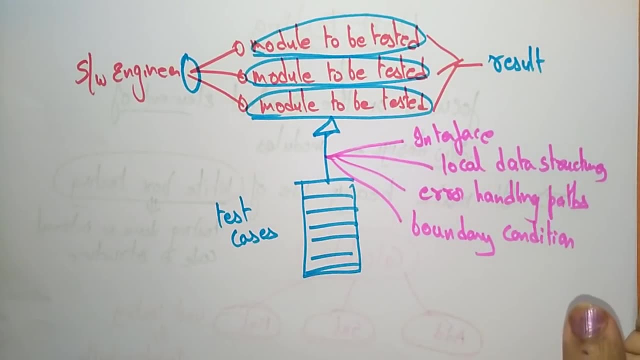 interfaces- the test case has to be checked- and the local data structures. the local data structure consideration here is it is going to check whether the incorrect variables, names is there or not, means is present, it inconsistent data types are there here or not? and underflow, overflow and addressing exceptions are erased. so that will be done. so based on the 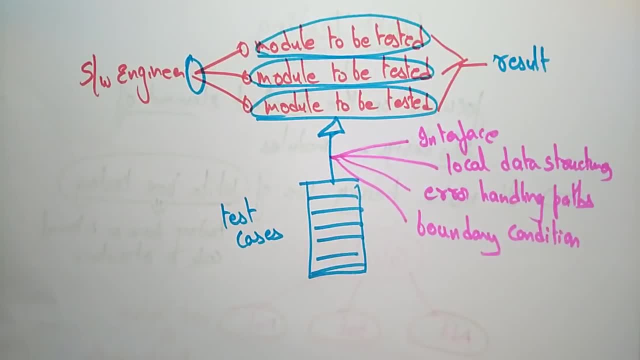 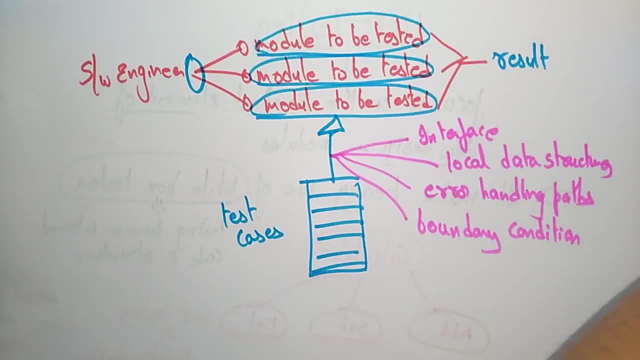 local data structures. the test cases will be done and it will be tested on each module. okay, and some, uh- error handling paths. whether it is checking all error handling paths will be how it is going to handle the error handling means the except exception handlings is incorrect. it is going to check whether the exception handling is incorrect.